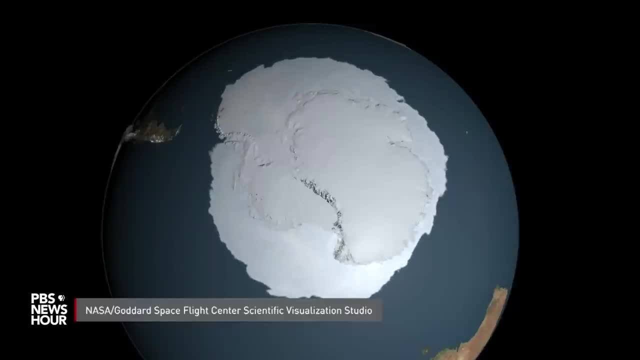 ocean. It doubles the size of the continent every single year, But the problem is is that this year and last year to a similar extent, that ice has not been growing nearly as quickly. I want to put up this other chart here. This shows the traditional. that line at the top is: 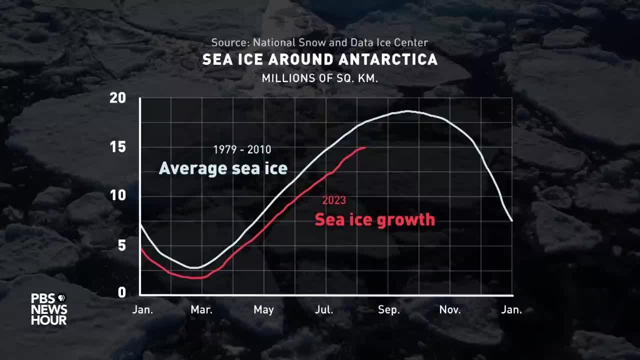 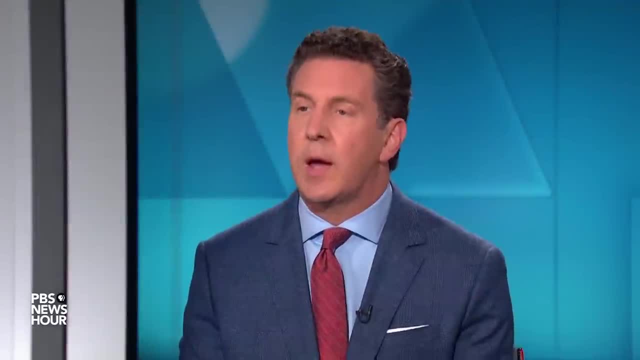 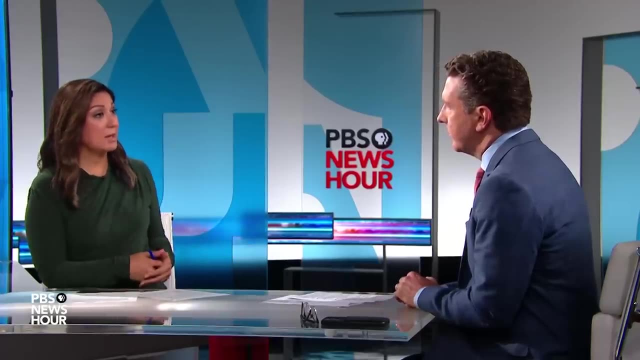 what normal growth of the sea ice is. That red line below is where we are now. It is a marked difference. That is roughly the size of Alaska. that is missing ice now in the Southern Ocean. That's remarkable to see in the graphic there. You have been talking to researchers. Do they know why this is happening? 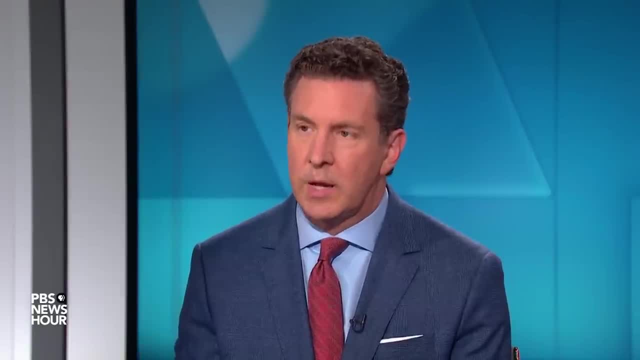 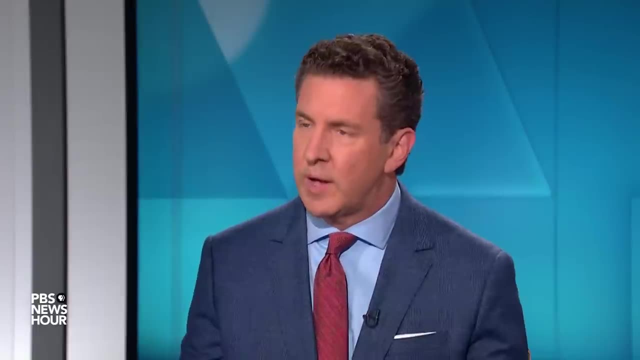 It is a complicated picture. There are some leading suspects. These are all suspects that we have our fingerprints on. The first one is that the ocean is warmer. We have seen that all over the world As we burn coal and oil and gas and warm the atmosphere. 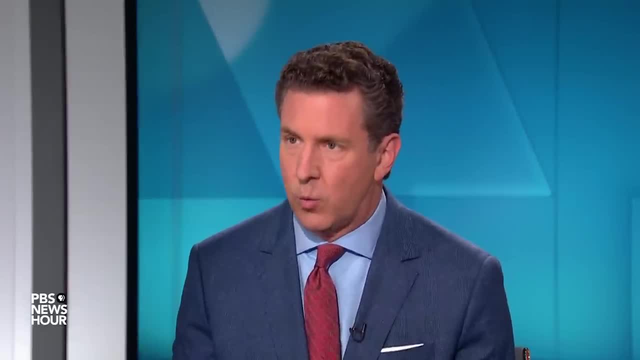 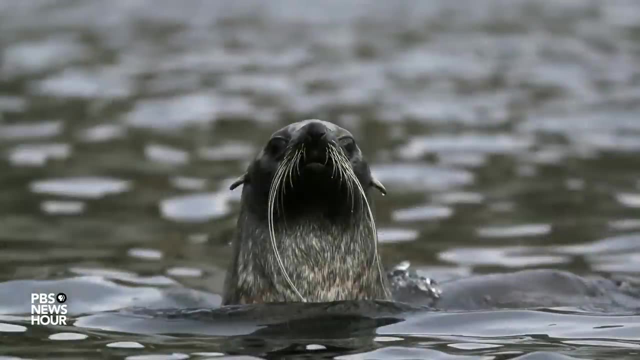 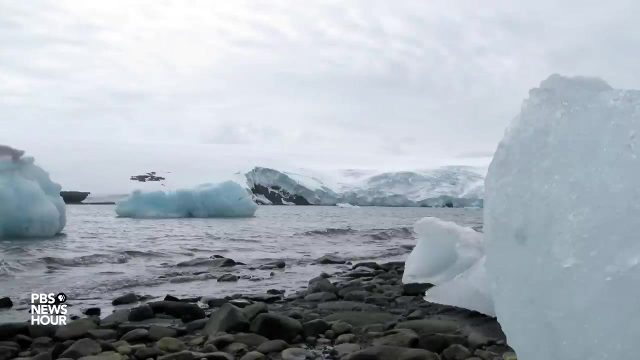 that warms this planet And the oceans absorb the bulk of that warming. Warmer ocean water makes it hard to grow ice. That's pretty standard physics. The air is warm as well. That makes it harder to grow ice. Wind is also complicit in this: changing wind patterns- Wind is really 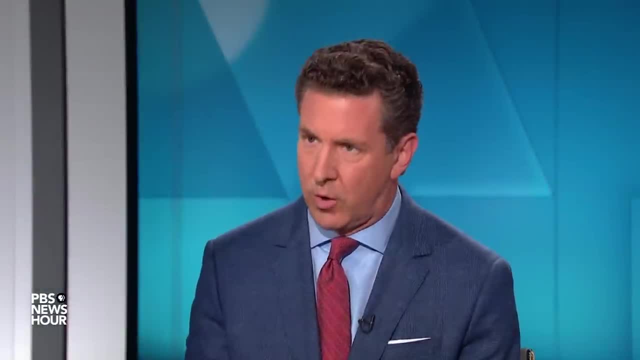 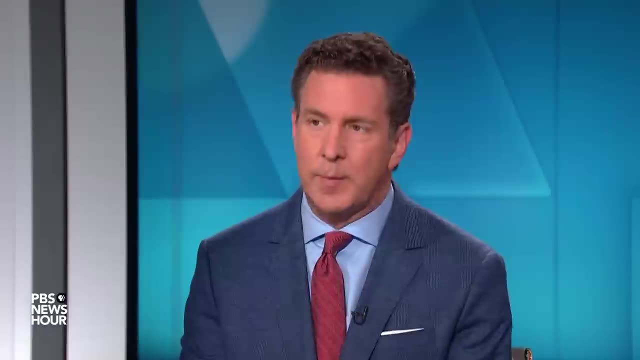 important in how ice grows off of Antarctica and where it grows. Those things are changing Again. scientists believe that we are one of the main drivers of this, but the exact mechanism is not totally clear. AMNA NAWAZ. So what's the bigger concern in all of this? 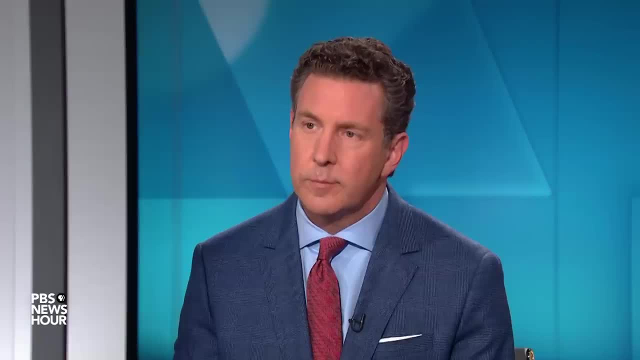 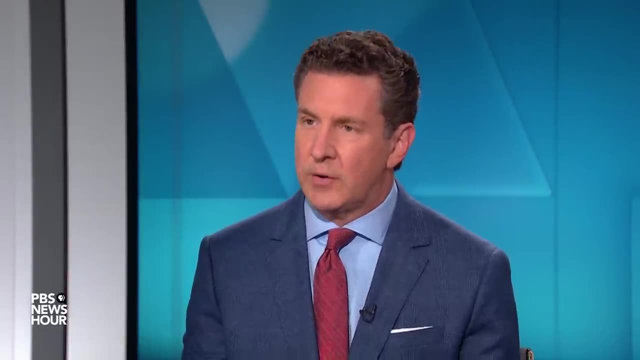 If that sea ice is not growing at the rate it's expected to, what are the consequences of that? DR ANTHONY FAUCI, This is the biggest issue here, And the reason we care about this is that that ice provides all sorts of incredibly valuable things for us. 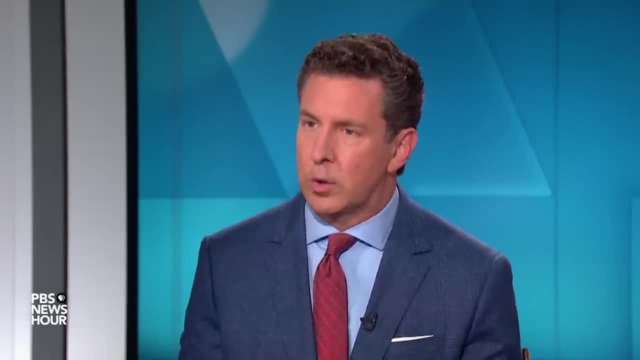 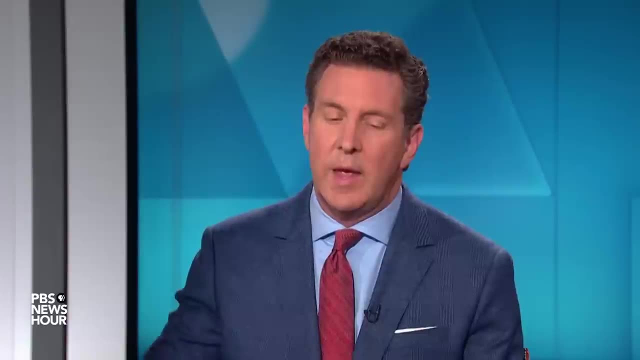 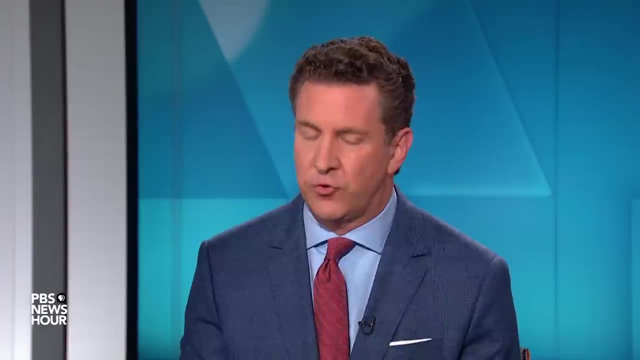 First off, that ice keeps the Southern Hemisphere cooler, And you think of ice as this flat white surface That reflects the sun's radiant energy off into space. If that ice is not there, that sunlight hits the ocean, warms the oceans. This is part of a very complicated engine that 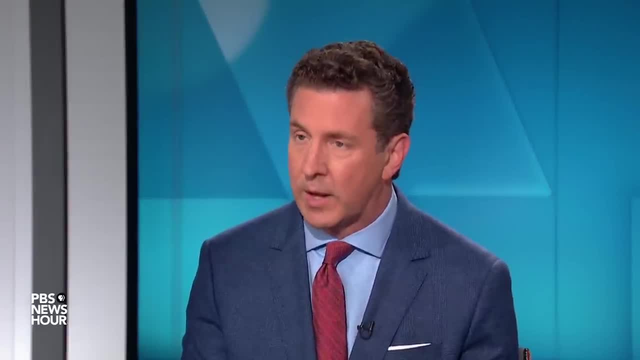 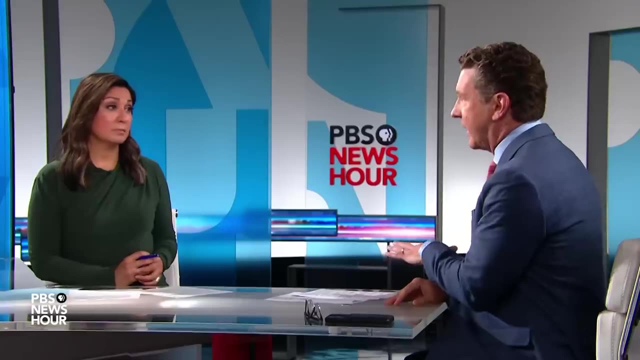 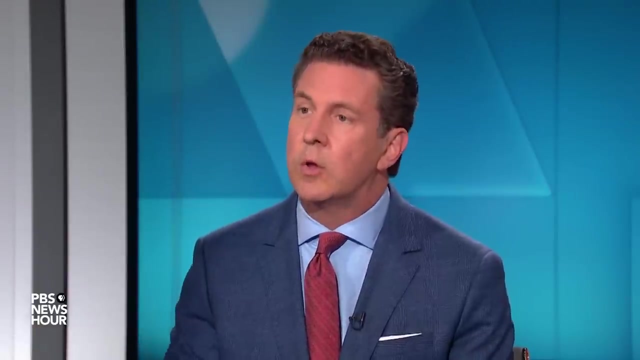 drives ocean currents globally and weather patterns globally, So disrupting that could cause huge problems. DR ANTHONY FAUCI, This sea ice also protects the glaciers that are sitting up on land in Antarctica. We want those glaciers to stay there If they slip into the ocean that raises sea level rise globally.